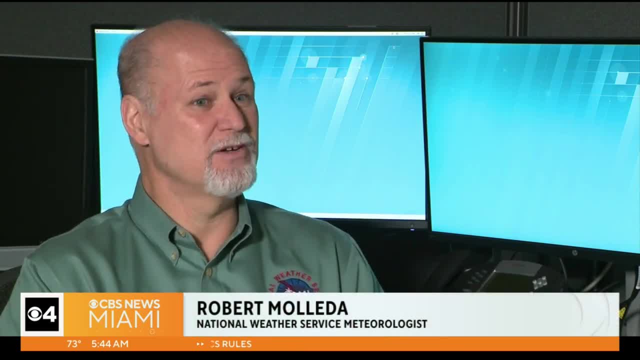 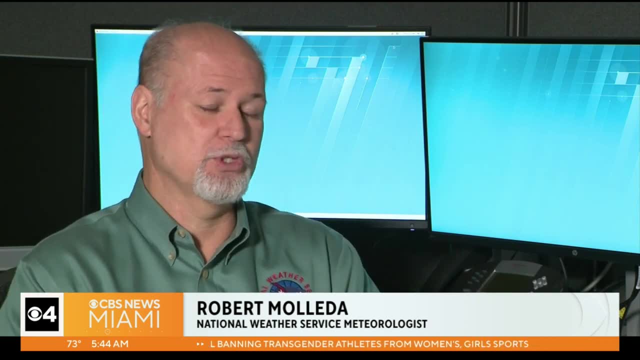 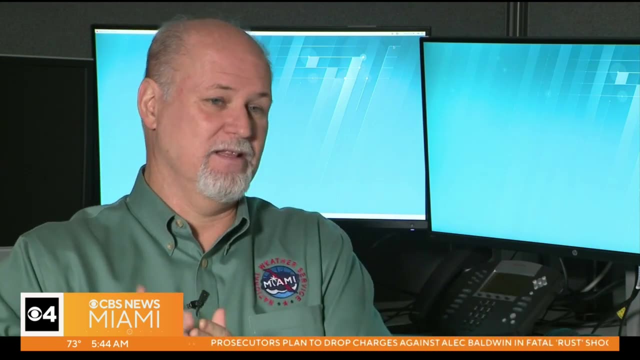 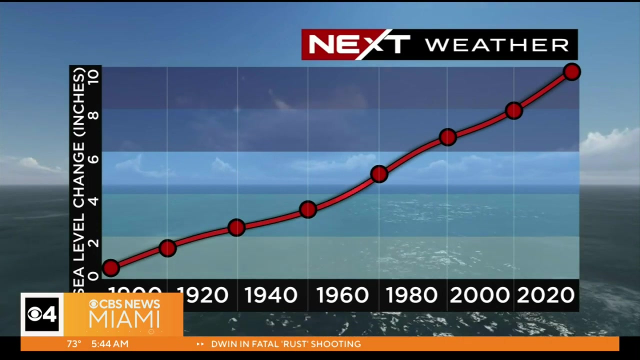 has changed by about three millimeters per year. Again doesn't seem like a huge deal, but if you average that, or if you extend that out over a course of, let's say, 50 to 100 years, we're talking almost a foot of a rate of increase over that, let's say, 100 year period. That's what the sea level data collected by the National Weather Service office in Miami shows: The rise not only occurring year over year, but it's also increasing. So that's what the sea level data collected by the National Weather Service office in Miami shows: The rise not only occurring year over year, but it's also increasing. So that's what the sea level data collected by the National Weather Service office in Miami shows: The rise not only occurring year over year, but it's also increasing. So. that's what the sea level data collected by the National Weather Service office in Miami shows: The rise not only occurring year over year, but it's also increasing. So that's what the sea level data collected by the National Weather Service office in Miami shows: The rise not only occurring year over year, but it's also increasing. So. that's what the sea level data collected by the National Weather Service office in Miami shows: The rise not only occurring year over year, but it's also increasing. So that's what the sea level data collected by the National Weather Service office in Miami shows: The rise not only occurring year over year, but it's also increasing. So. 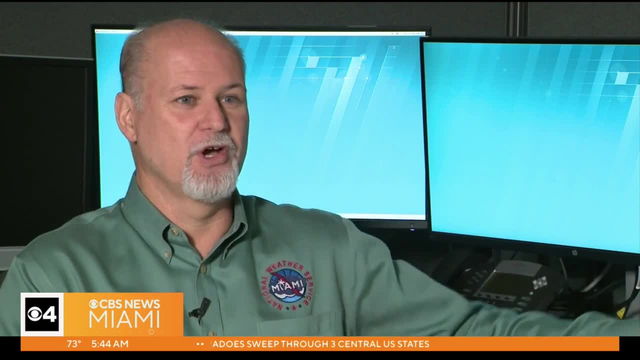 that's what the sea level data collected by the National Weather Service office in Miami shows: The rise not only occurring year over year, but it's also increasing. So a weather event that maybe 30,, 40 years ago would not have caused some tidal flooding. 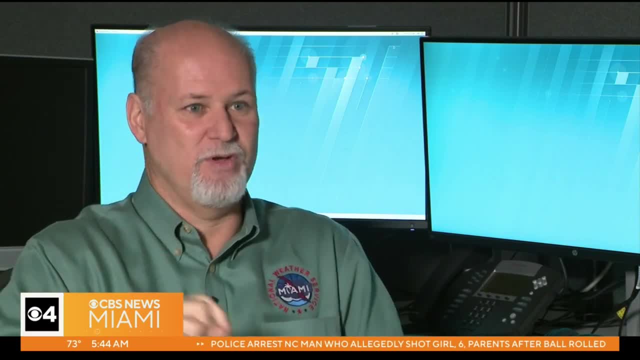 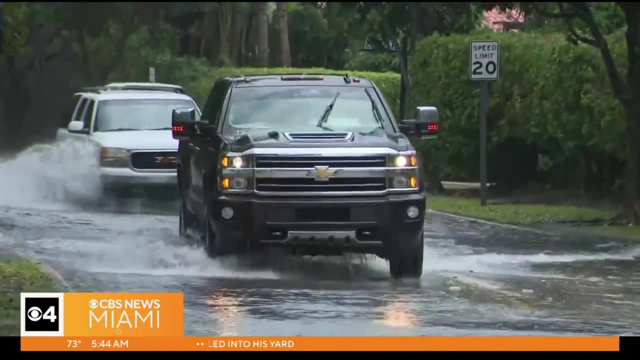 Just that those extra few inches could make the difference between no flooding and some water getting up over seawalls, or maybe water- you know, groundwater- seeping up a little bit higher, closer to the ground. The reality for now is that South Florida will continue to see. 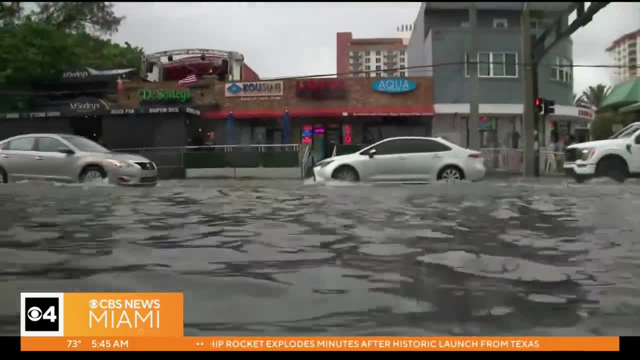 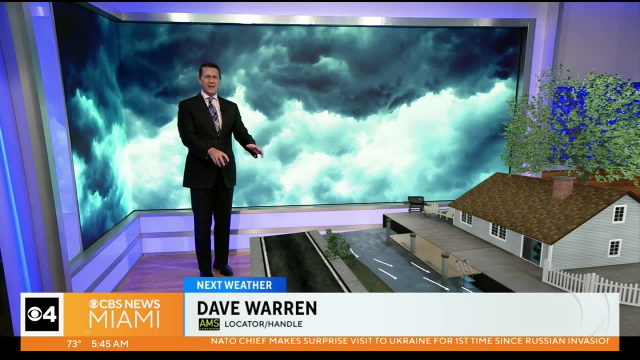 increased impacts along the coast, inland and even underground. Well, this is the typical setup: road and the houses next to these canals which force the water out to sea. That's how we get rid of these floodwaters. along the coast, and also over the interior, You get some heavy rain, Typically. 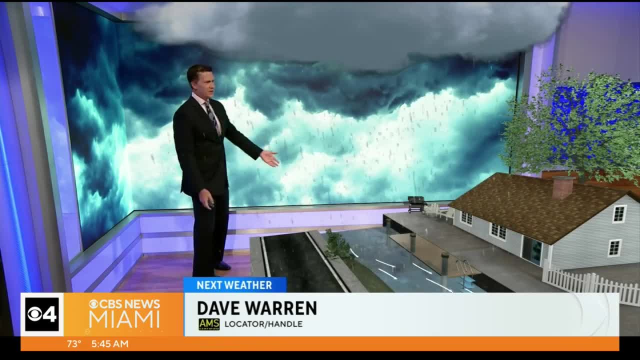 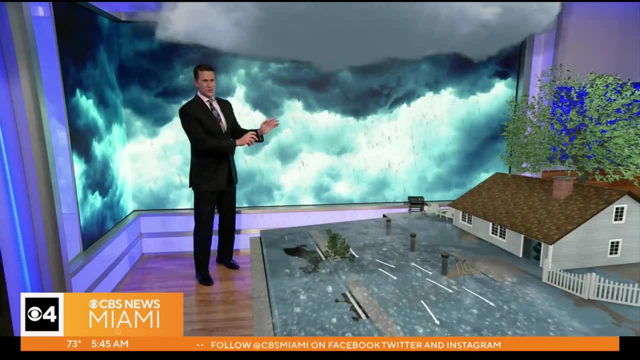 you see some minor flooding in and around the areas here. There's the rain coming down. The waters rise a bit. Now what's been happening recently is, with the heavy rain and the increased sea level, this drainage does not happen as quickly as it normally would. You have less. 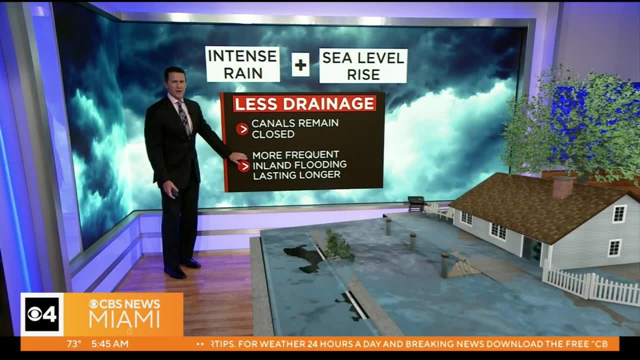 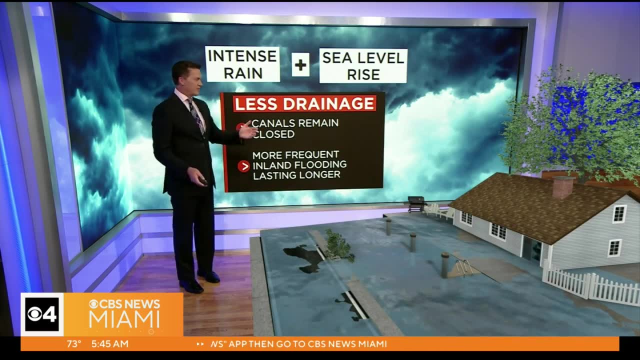 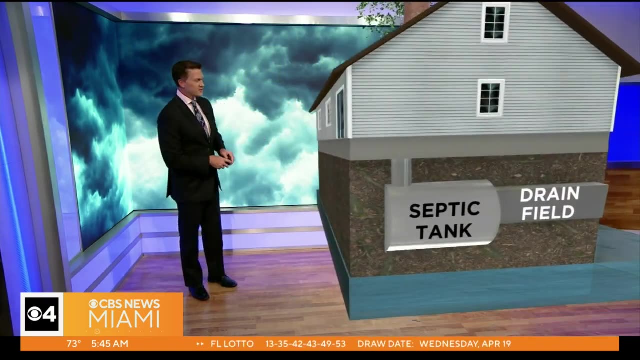 drainage because of intense rain and sea level rise. More frequent episodes of this flooding are occurring now because the canal gates remain closed for a longer period of time, So this is likely to continue here. What else is happening is underground. A number of houses here in South Florida have septic systems. This is how it should.